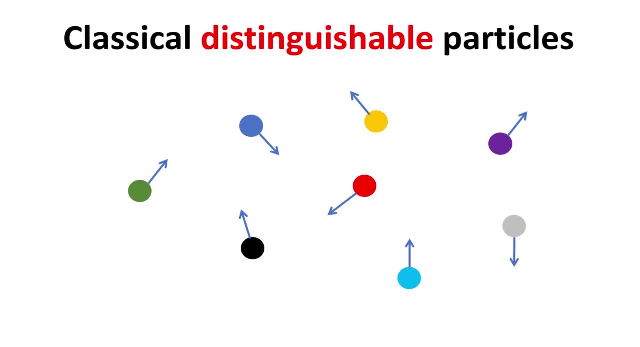 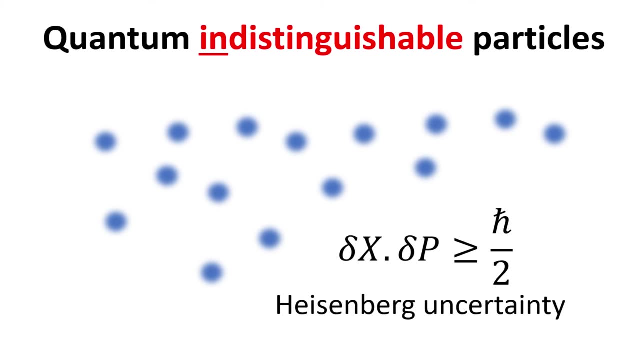 time is deterministic, thus allowing us to effectively label each particle, like how I do it here with the different colors. With the understanding of quantum mechanics, we now know that truly classical microscopic particles don't really exist. Microscopic particles are described by wavefunction whose position and velocity cannot be determined. 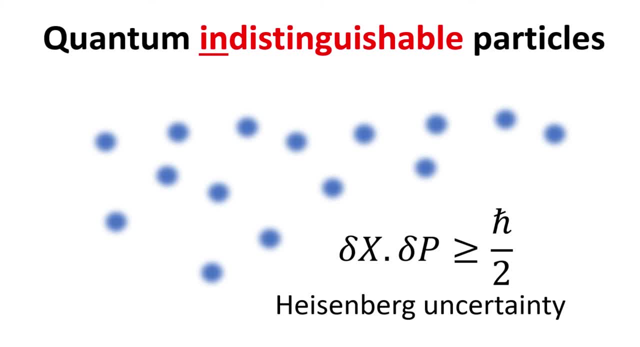 simultaneously A fact known as the Heisenberg uncertainty principle. Such fuzziness in their position and momentum dictates that quantum particles cannot be distinguished from one another, which has important implications on their statistical distributions. Hence quantum particles are indistinguishable from one another, such that there is no way we 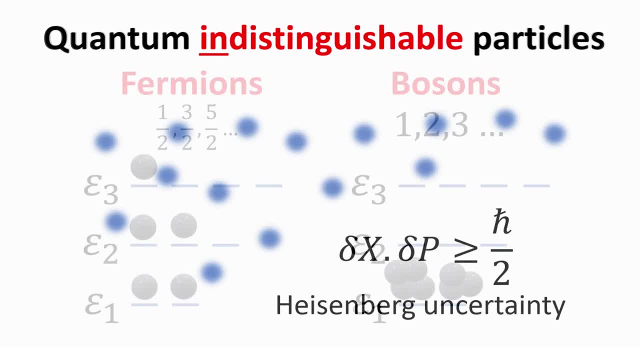 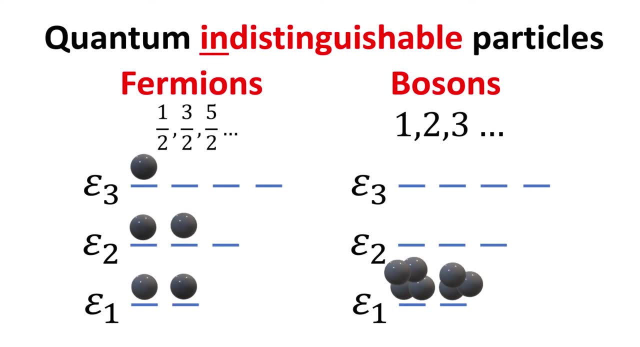 can label them individually with different colors, like in the classical counterpart. There are two types of quantum particles, namely fermions and bosons. Fermions have half-integer spin and satisfy the Pauli exclusion principle, which requires a maximum of only one fermion per quantum state. Bosons, on the other hand, 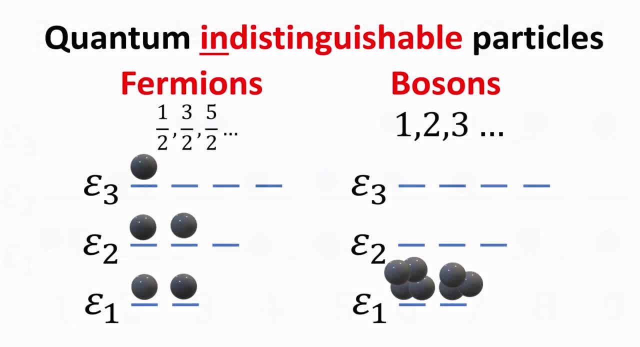 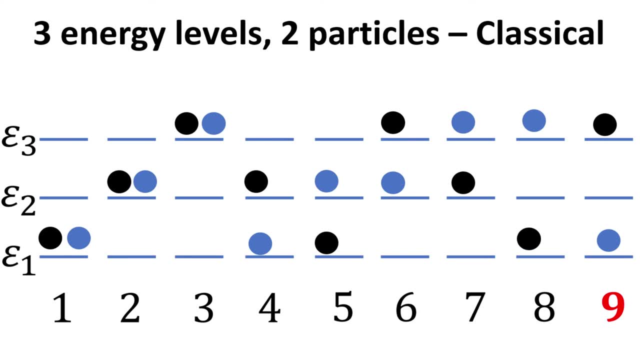 are integer spins and do not need to comply with the Pauli exclusion principle. As an example, let's consider a system of three singly degenerate energy levels and a total of just two classical particles. Since classical particles are distinguishable, we label them with different colors. One can see that there are a total of nine different. 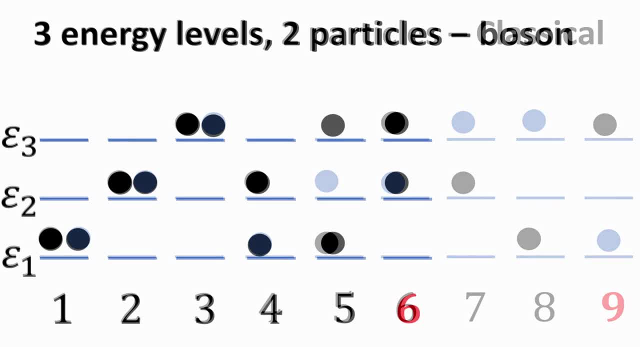 ways of distributing these two particles across the three levels. Now let's consider the quantum particle boson. In this case, bosons are indistinguishable quantum particles, so we denote them with the same colors. The number of ways of arranging them are six. 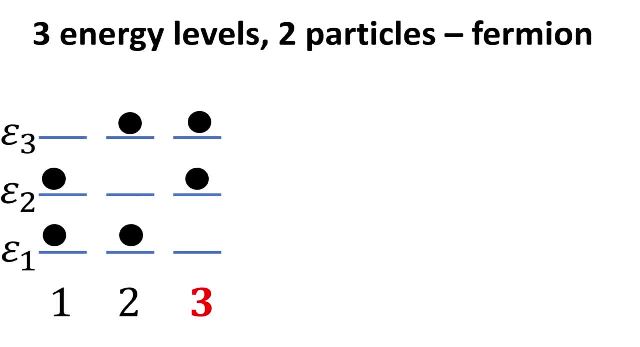 Lastly, let's consider the quantum particle fermion. In addition to being indistinguishable quantum particles fermions also have to respect the Pauli exclusion principle, so we cannot populate more than one fermion in any energy level. This severely constrains the number of arrangements. 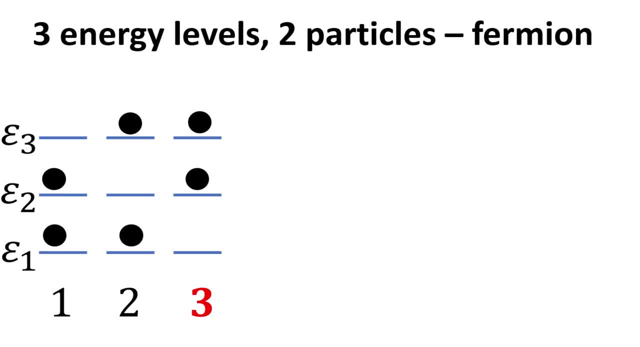 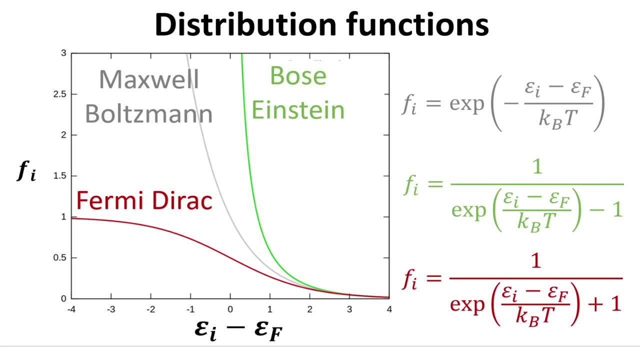 and we arrive at the same number of fermions. To conclude, we show here the shape of these distribution functions plotted against the difference of the energy with respect to the Fermi energy. The Fermi-Dirac occupation is half when at the Fermi energy and approaches one and zero when